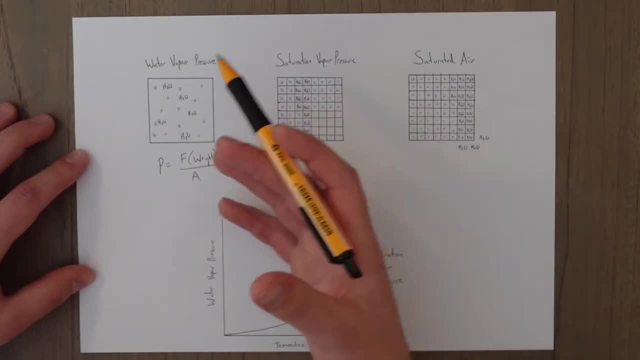 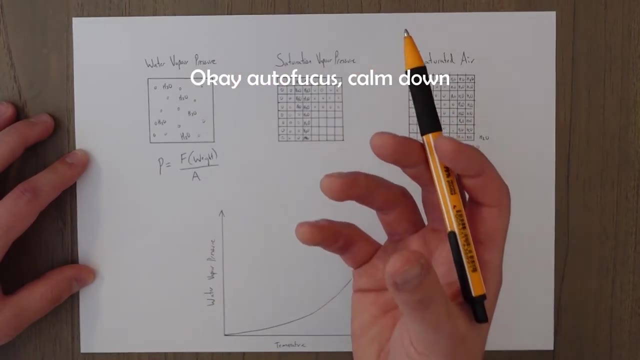 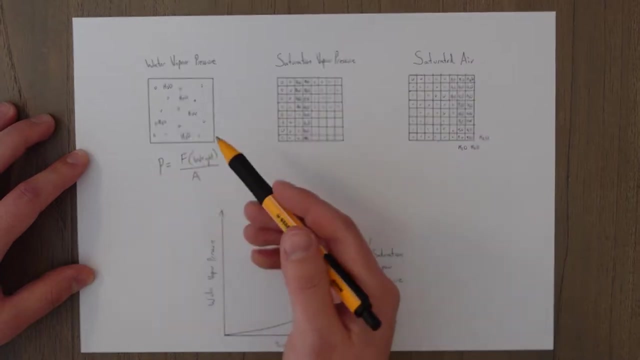 which it exerts onto the air molecules and the air around it. Pressure can be kind of a confusing term, because it's more like the amount of water vapor that is in the air, but because it has a weight which is a force, and it's exerting that over certain areas, you can think of it as a. 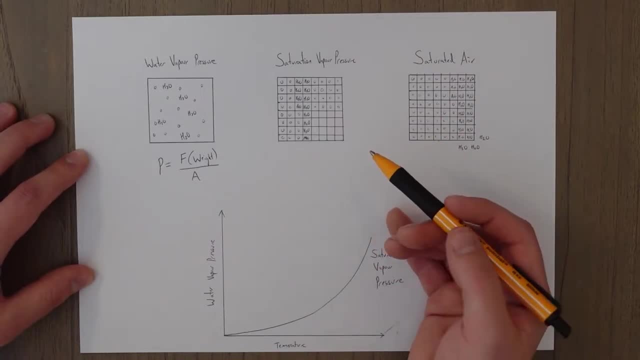 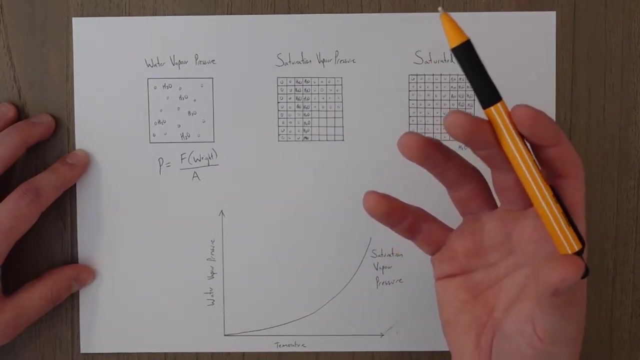 pressure, because pressure is force over area. The air has a fixed amount of water which you can hold, which I have represented here by this grid. If you think about each molecule taking the up one square of this grid, there's only a certain amount of squares before there is no more room. 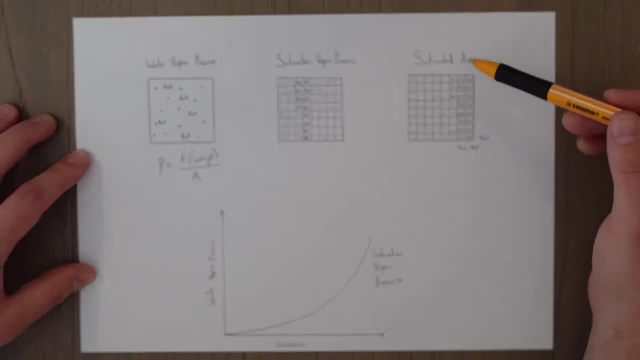 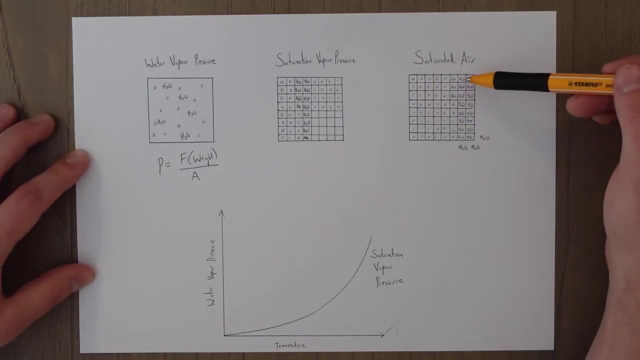 which is what happens when we've got saturated air. You can see all these squares are filled in. we've got regular air molecules- nitrogen, oxygen, trace gases- and then you've got the water molecules in the air and it gets full, and then any more water molecules are then condensed out into liquid form, So you've got water vapor. 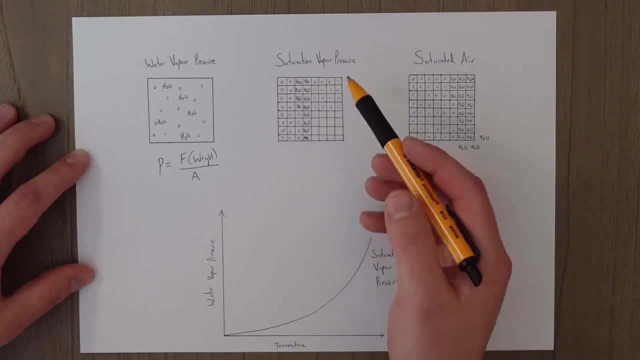 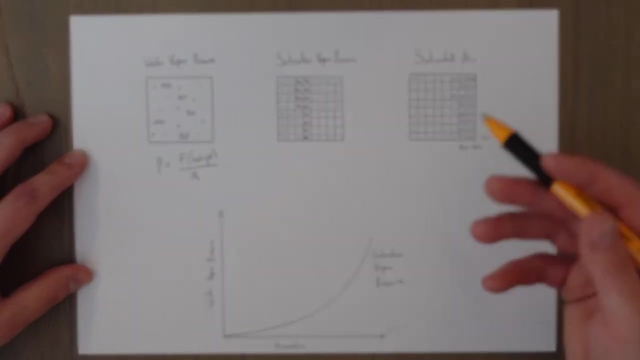 which is the amount of water in the air. Saturated vapor pressure is the amount that it can hold, and the saturated air would be when the water vapor pressure and the saturation vapor pressure are equal, and then any more water that is added in condenses out and forms liquid, and 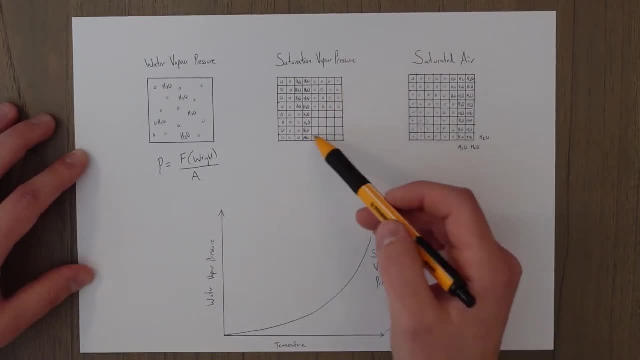 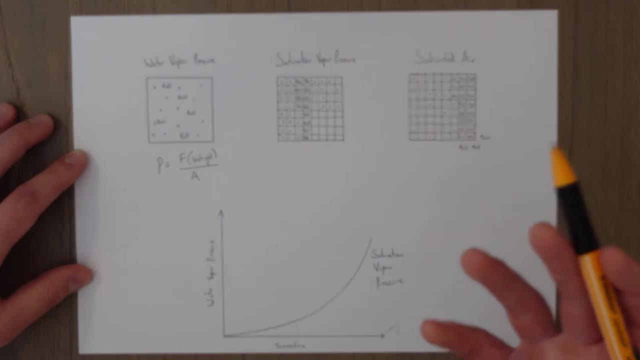 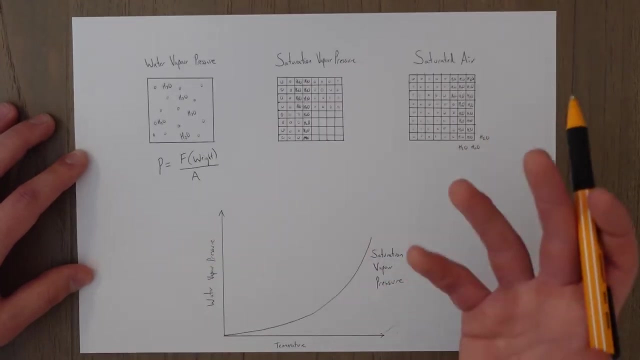 clouds in essence. So the saturation vapor pressure, this grid, varies according to the temperature. Basically, what happens is energy in the form of heat is used to break the chains of liquid water molecules apart into the individual molecules, which is what water vapor is. If the air is warmer, then there is more energy and the air can break these chains of. 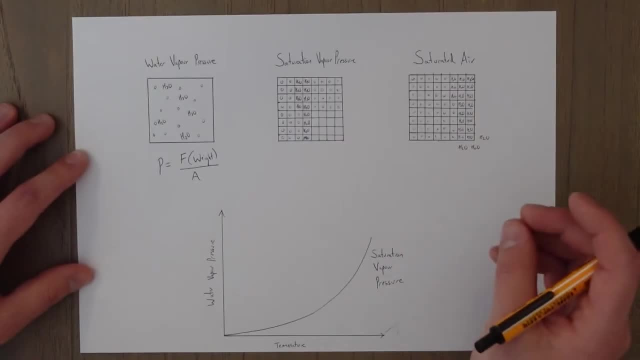 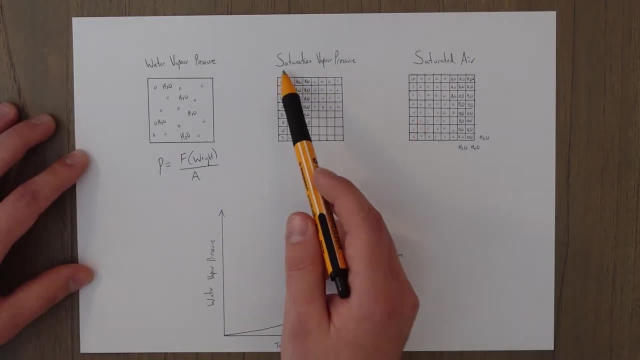 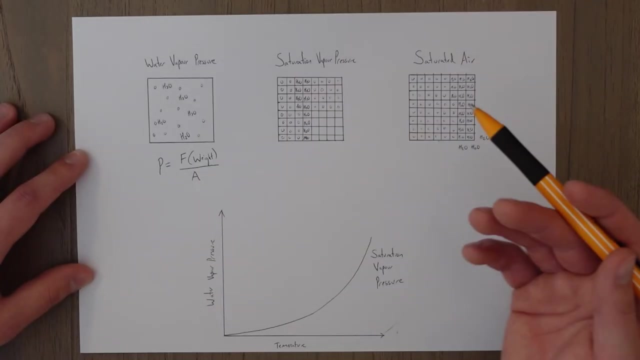 molecules into individual, separate molecules more easily. What this means in practice is that warmer air can hold more water vapor. It has a higher saturation vapor pressure than cold air. This, in essence, is the theory behind cloud formation. The water vapor rises into colder air and the saturation vapor pressure comes down to meet. 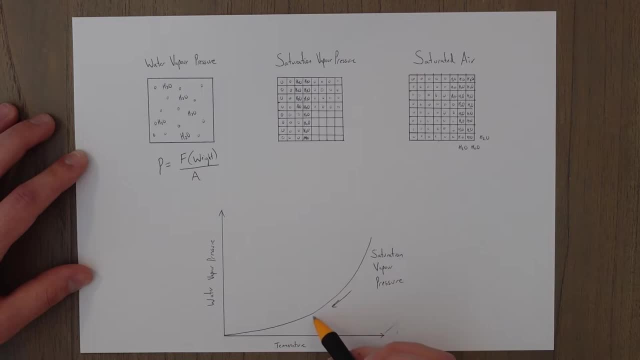 the level of actual water vapor pressure in the air and it condenses out and starts to form clouds. Another way to think of saturation vapor pressure is if you have like a towel and you're wiping up some water, You can only wipe up so much water before the towel becomes. 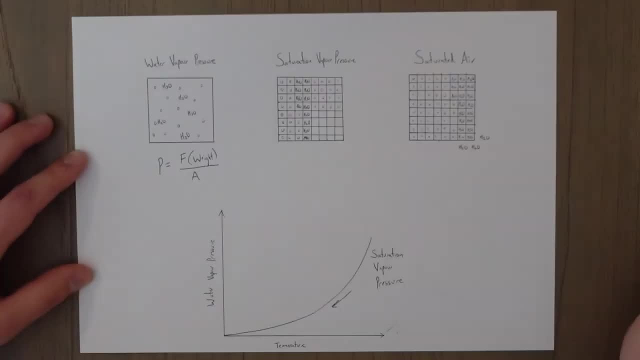 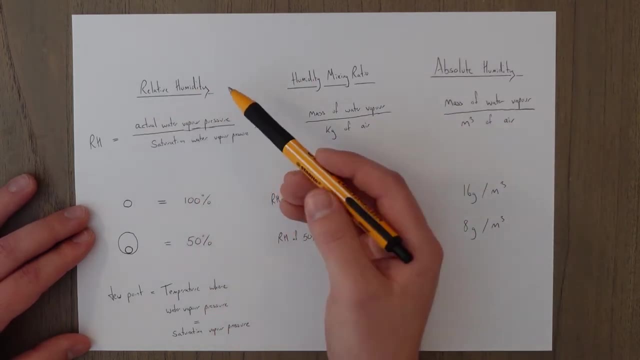 saturated and any more water just leaks out of the towel. There's a few different flavors or types of vapor, love of illegality. we've covered so far and i'd like to look at some in that context. Of course, we do want to talk about the role of saturating. 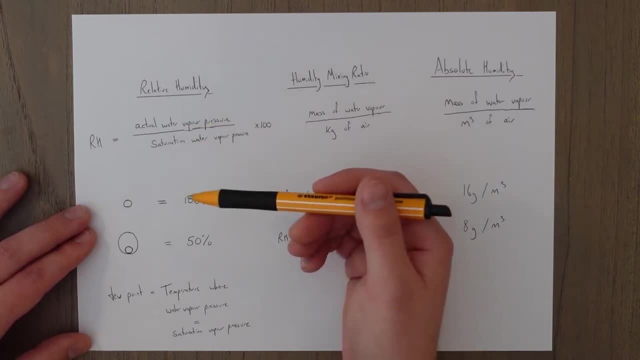 So, similarly, you can plug and speakerãy different types ofpersonal category vapor in cutter as well. In this case we're talking about the air vapor pressure that if you select in the Scandinavian paper. So let's start with the most common type that we have is relative humidity. this is the amount. 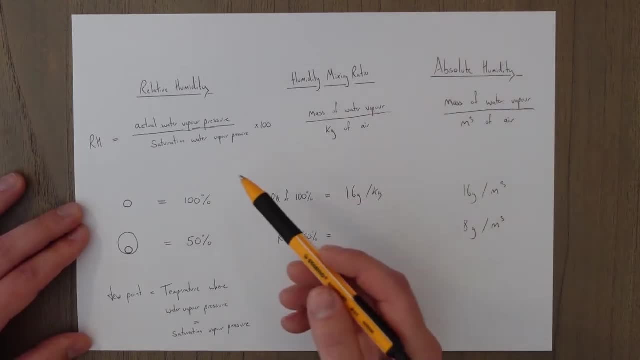 of water vapor in the air compared to the max that the air can hold as a percentage. so it's the 1 actual water vapor pressure, the water vapor in the air compared to the saturation water vapor pressure. we divide one by the other and then we multiply by 100 to get percentage. so as the temperature changes, the 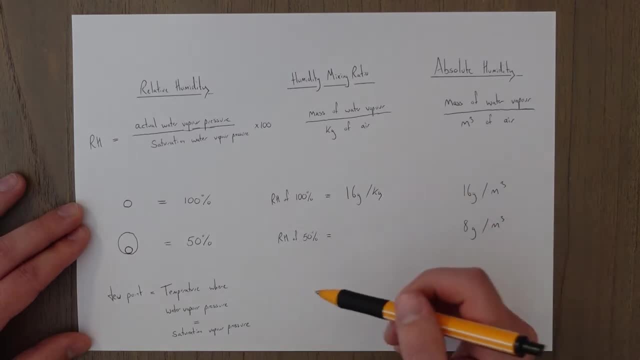 saturation vapor pressure will change as well, which will have an impact on the relative humidity, so that we can actually have an impact on care humidity. that was that graph with the line we saw earlier. as it gets hotter, the amount of saturation vapor pressure will go up. we can hold more water in the air, which means that if we have the same 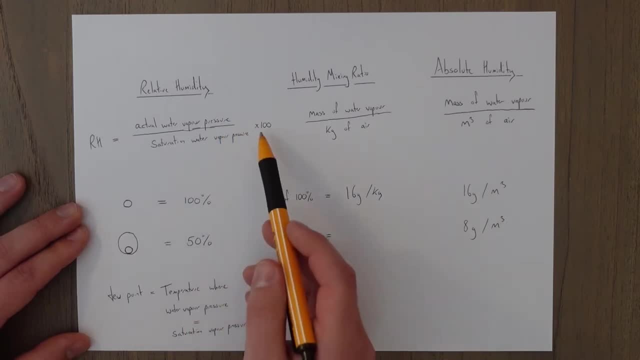 actual vapor pressure, but we get warmer, the relative humidity will change. think about this as being the 100. we would have the actual water vapor pressure and the saturation water vapor pressure is the same. it'd be the same amount, but then, as we get warmer, the saturation water vapor pressure will increase, but the actual water vapor pressure remains the same, so our relative humidity will go down. there's a phenomenon called a dew point, a temperature called a dew point, which is the temperature of air where the saturation vapor pressure and the water vapor pressure are exactly the same. 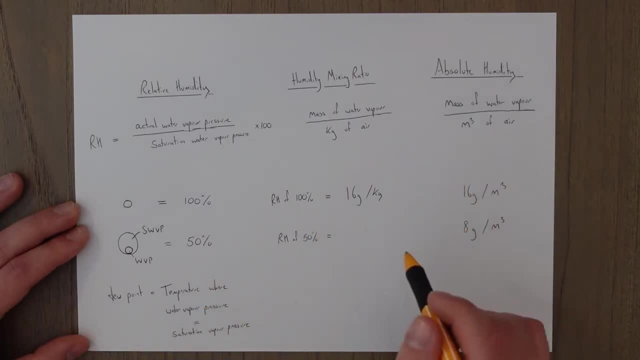 what happens is that line that we saw reduces down until the saturation vapor pressure matches the actual water vapor pressure and clouds start to form. the water starts to condense out. you can think of it as, basically, where the relative humidity becomes a hundred percent. the humidity mixing ratio describes how many grams of water vapor are held within a specific kilogram of air. as air increases in temperature, it will be able to hold the same amount of water vapor and the air will be able to hold more grams of water per kilogram. the saturation water vapor pressure will go up, which means more water vapor molecules can come in and therefore the weight increases. 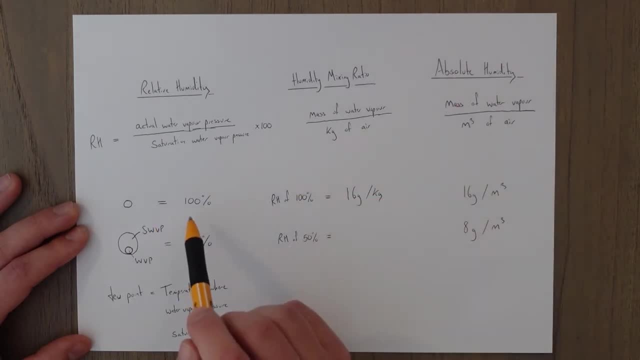 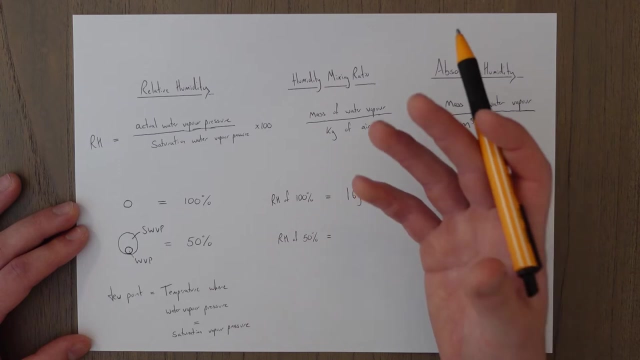 we can say that this mass of here, whilst having a relative humidity of 100 percent, has a humidity mixing ratio of 16 grams per kilogram, for example. note that 100 percent of relative humidity doesn't mean that all of the air is water. it means that it's a hundred percent saturated. that's what I like to think of it, as it's a 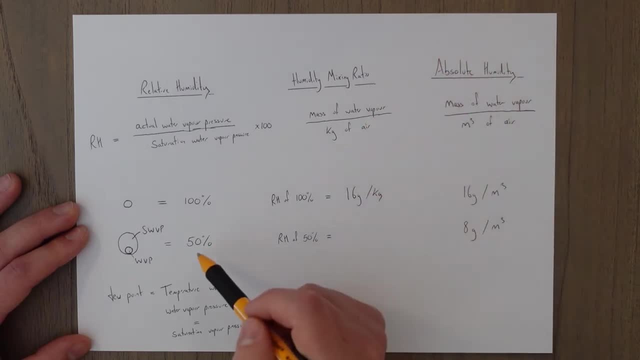 percentage of how much air would take to saturate. so that's 50 of the way to being saturated, that's 100 of the way to being saturated. so in this case, with a relative humidity of 100, we've got 16 grams per kilogram. we could imply that a relative humidity of 50, we'd have eight grams per kilogram. 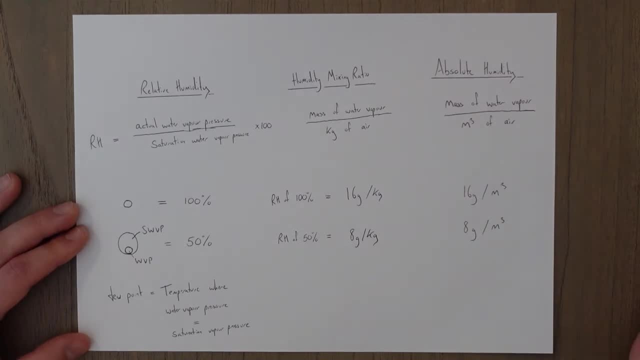 that would be our humidity mixing ratio. absolute humidity is we take the mass of the water vapor but then we compare it to the volume of air. it's kind of like the water density in the air and it will vary a lot with geography of where you are. somewhere close to sea is bound to have more water in the air per cubic meter than 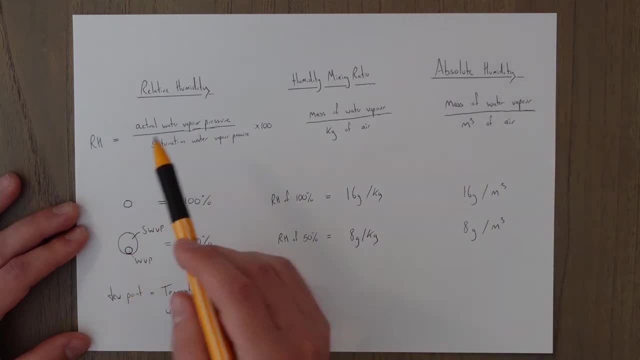 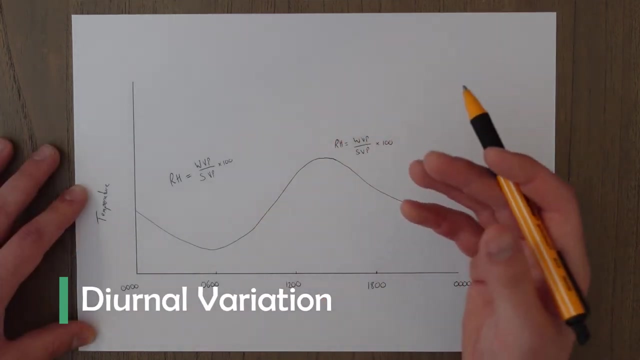 in the desert, for example. so whereas relative humidity is the level of saturation in the air, the absolute humidity is a very quantifiable amount. it's the mass of water per volume, and so is the humidity mixing ratio. mass per kilogram. diurnal variation is a fancy way of saying the date night. 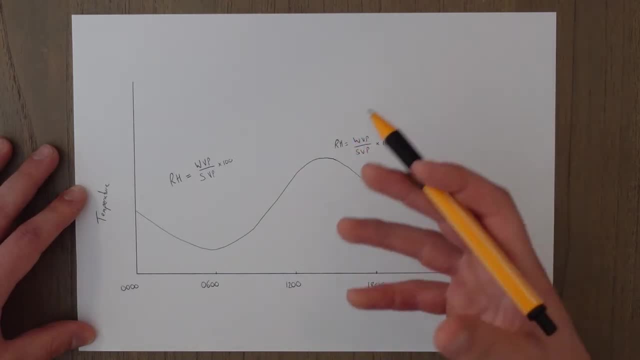 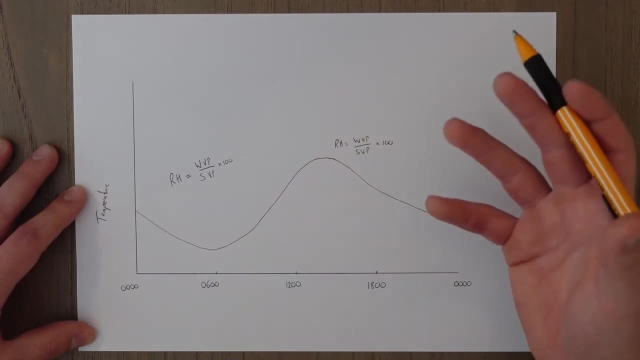 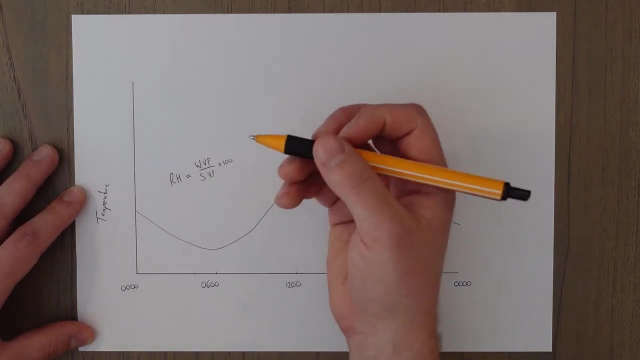 cycle. so the influence of the sun and the heat it gives off in terms of temperature influence the relative humidity. basically, it gets cold at night and that influences what happens to the relative humidity. so if we take the nighttime example, this means that the saturation vapor pressure also changes. remember, warmer air can hold more water before 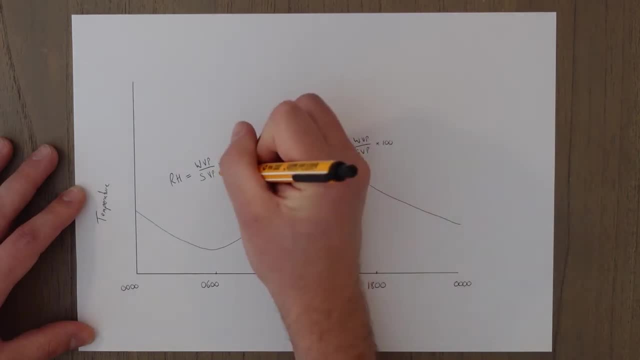 coming saturated, the value for saturation vapour pressure reduces. So if we have the same amount of water vapour pressure, that means that we're dividing by a smaller number and that sends the relative humidity up. So at night, if we have the same amount of water vapour pressure, the saturation vapour 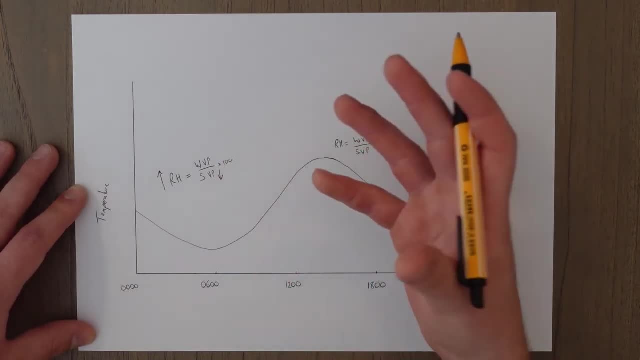 pressure comes down and makes it more relatively humid. And then the converse happens during the day, So the saturation vapour pressure goes up. we heat up the air, we can hold more water. So if we have the same amount of water vapour, we're divided by a bigger number, which makes 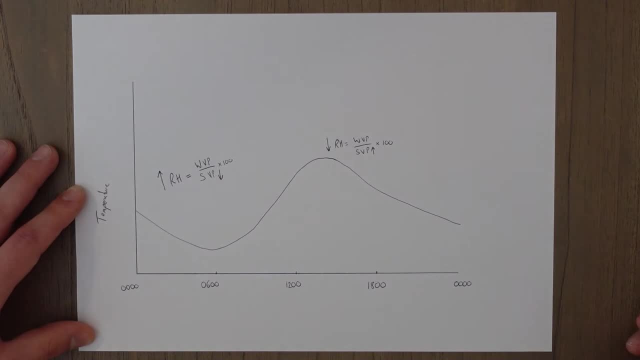 our relative humidity smaller, So it forms a line that looks something like this: As the temperature reduces to the dew point, the saturation vapour pressure reduces and we would get a relative humidity of 100%, And this is where the water vapour would condense out into forming clouds. 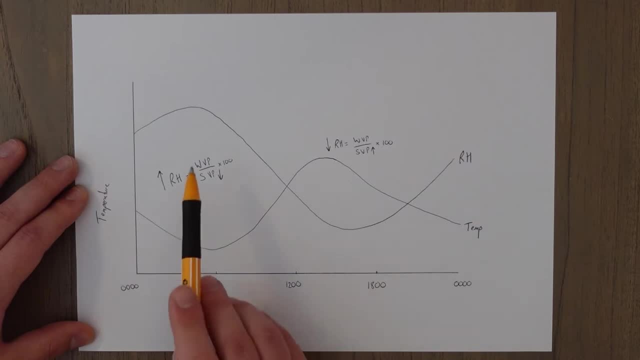 So at night, As the temperature is reducing, the relative humidity can shoot up, shoot up and if it reaches 100%, we start to condense out and form clouds, even if we're at the surface, And this is what fog and mist is. 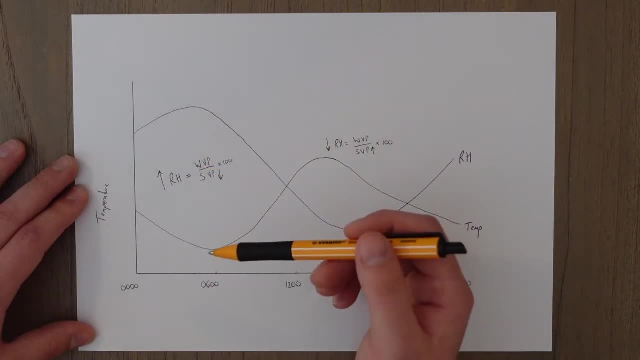 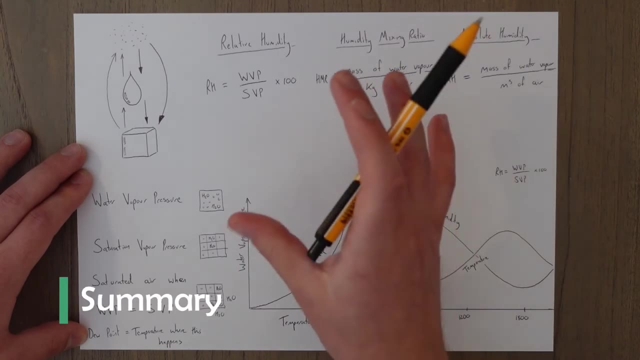 And this happens at the coldest point of the night, which is just before sunrise, And that is why you sometimes get early morning fog forming if it gets particularly cold at night. To summarise them, we've got the water cycle, we've got the gas, liquid and solid. 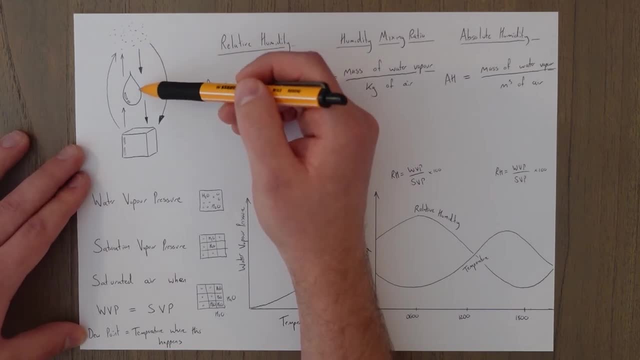 If we move from gas to liquid, we are condensing. If we move from solid to liquid, we're melting, then evaporating. If we move from solid to liquid, we're melting, then evaporating, And if we skip the liquid in the middle, we sublimate. 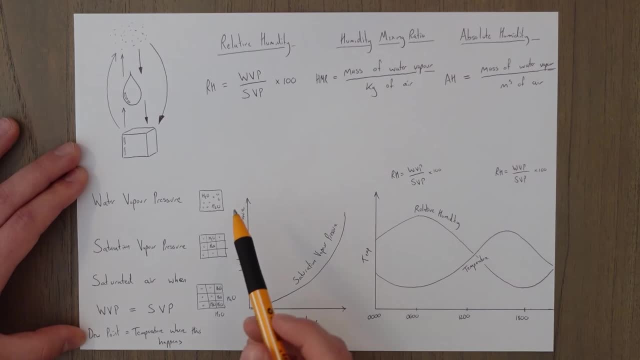 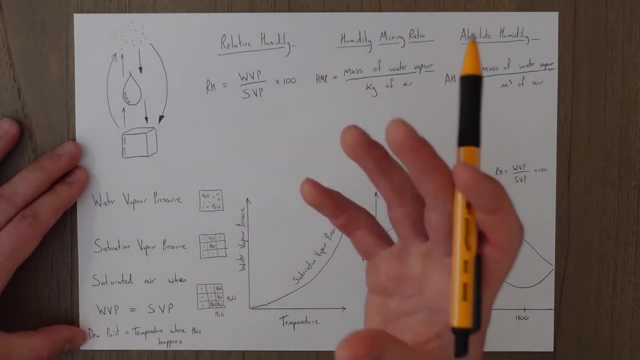 Sublimation between the two. The concept of humidity relies a lot on water vapour pressure and saturation vapour pressure. Water vapour pressure is the amount of water in the air. Saturation vapour pressure is the amount it can hold. That's the grid that I was talking about. 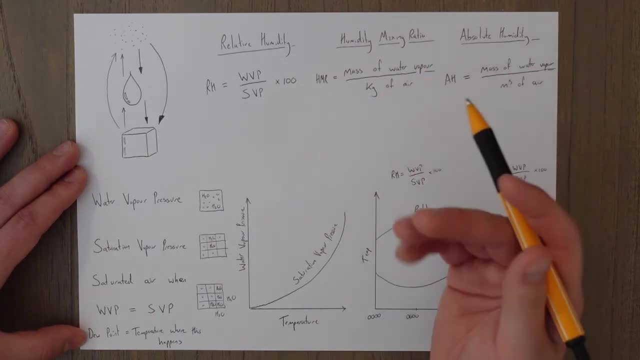 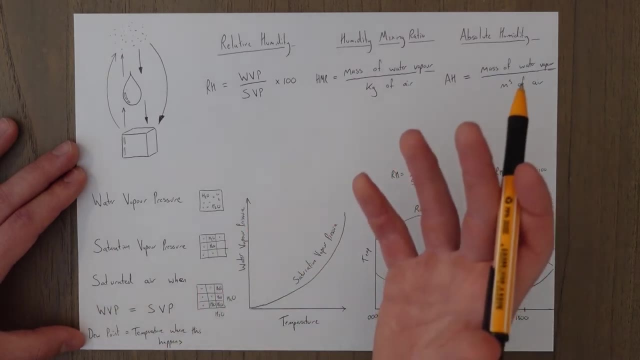 Or you could think of it as a towel. A towel could hold a lot of water. A towel can only hold so much water. Once this grid is full, or once that towel is completely wet, it is saturated. It can't hold anything else. And any more water will start to condense out and form liquid. The saturation vapour pressure varies with temperature. If it's hotter, we can hold more water in the air in the form of water vapour, And if it's colder, we come down and we can't hold as much. 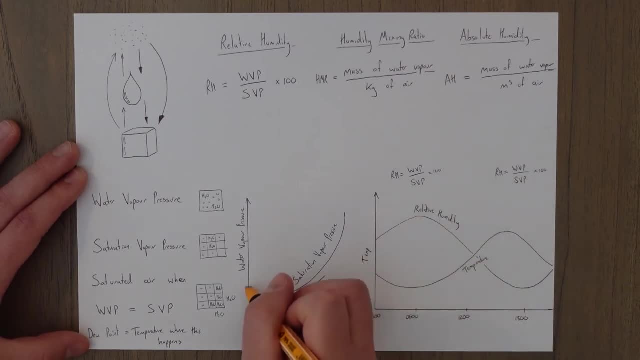 When the temperature reduces to the point where our actual water vapour pressure and our saturated vapour pressure are equal, we get to the point which is known as the dew point, And this is where the water vapour pressure equals the saturated vapour pressure. 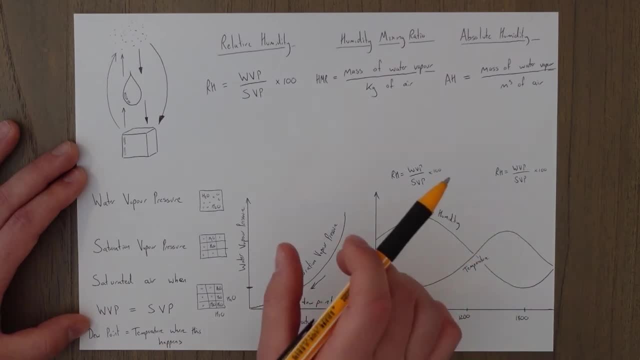 This is the basis behind cloud formation. You get water vapour rising, it starts to cool down and the saturation vapour pressure comes down to the point where the amount of water in the air, the water vapour that is rising, is equal. It goes into air where it can't be held any more, and it starts to condense out and form clouds. There's a few types of humidity. The most common one you see is relative humidity. This is the amount of water in the air compared to the amount that it can hold. 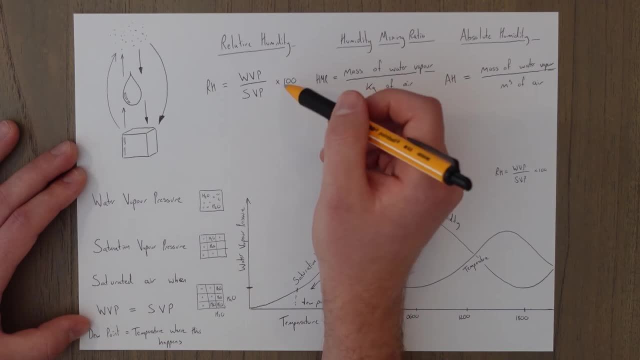 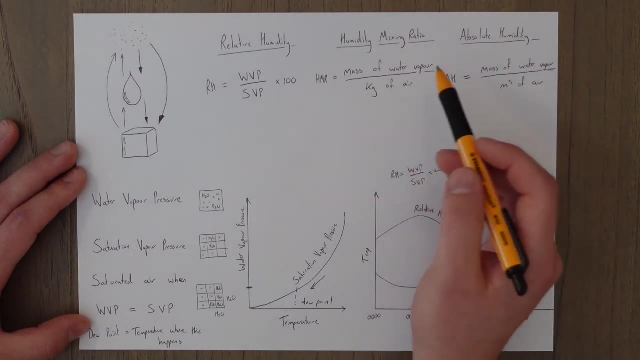 Water vapour pressure divided by the saturation vapour pressure, and then you multiply that by 100 to get it as a percentage. The humidity mixing ratio is the mass of water vapour per kilogram of air, a quantifiable amount, And the absolute humidity. I think of it as the water vapour density because it's the